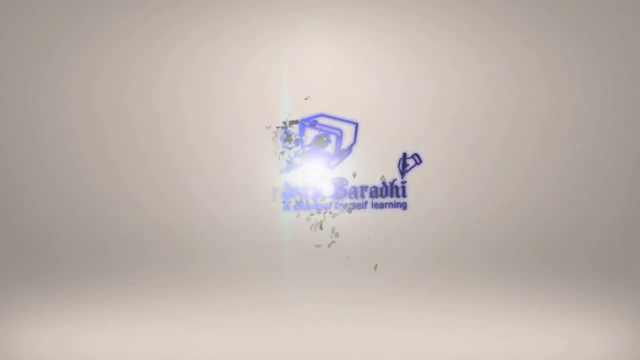 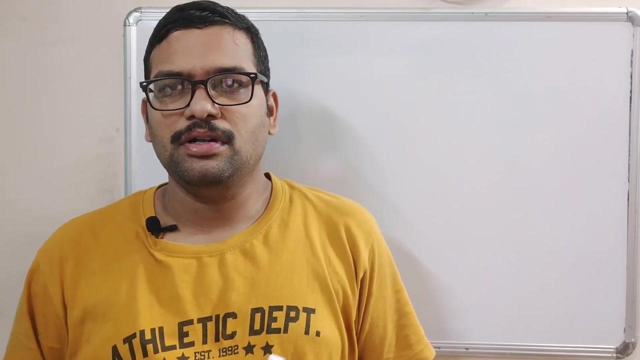 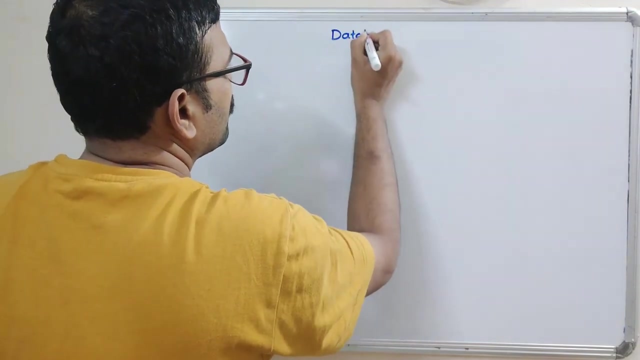 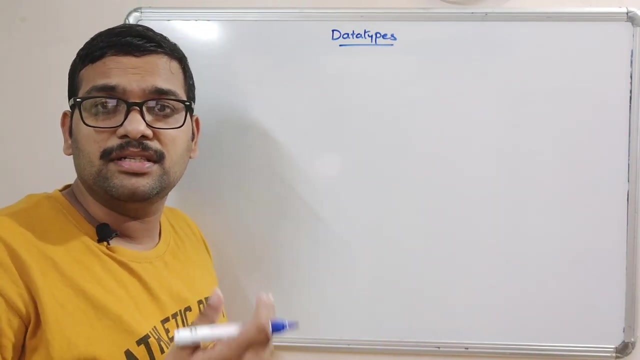 Hello friends, welcome back to our channel. So in today's session we will discuss about different data types available in JavaScript. So data type means so in other programming languages. this data type is very important because so we have to declare the variable. 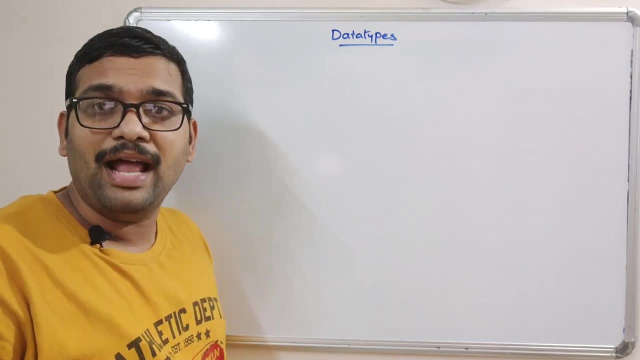 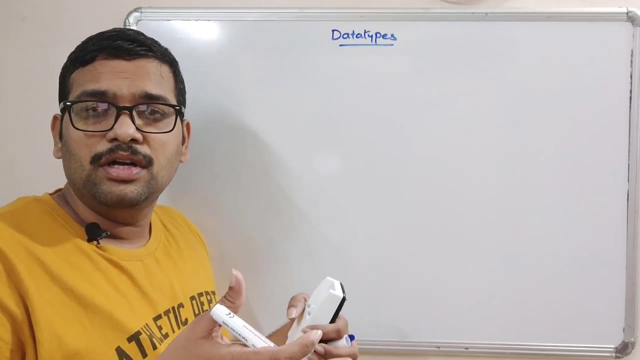 in one particular data type depends upon the value which has been initialized to that particular variable right. So if a variable holds the integer value, so we have to declare that particular variable using integer data type. If the variable holds the string value. 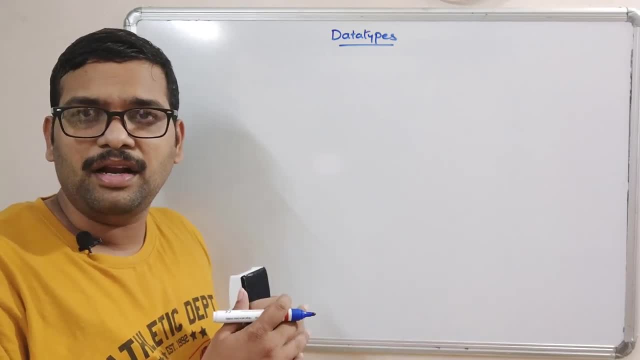 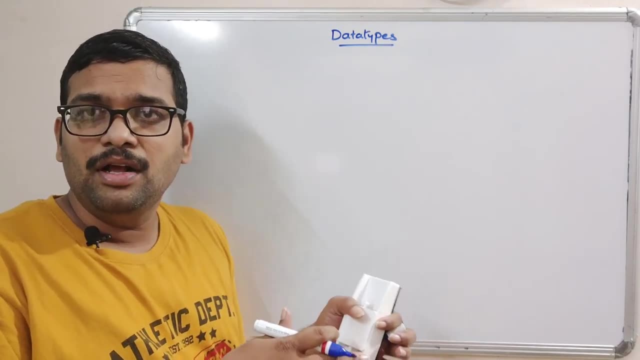 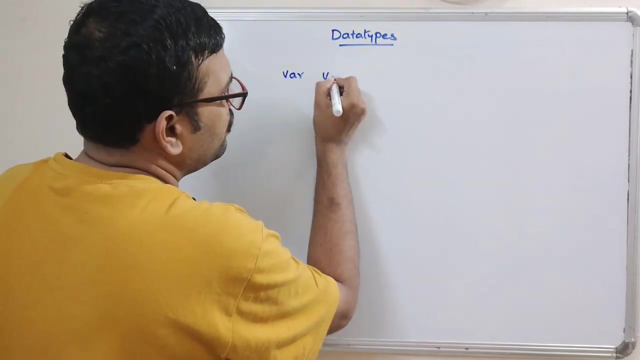 we have to declare using some character data type, right? So here, whatever the data type, that means, whatever the value we are storing into the variable, all the variables should be declared using only one keyword, that is, var, var, followed by variable- 1 comma variable. 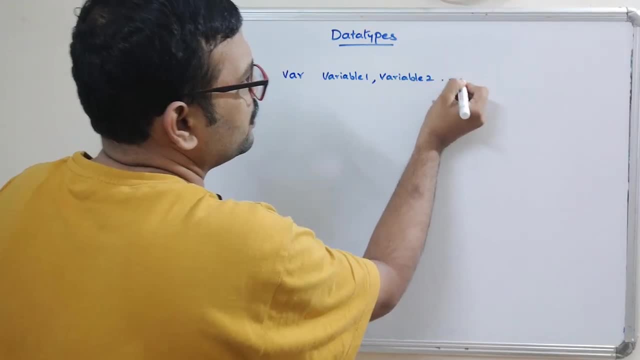 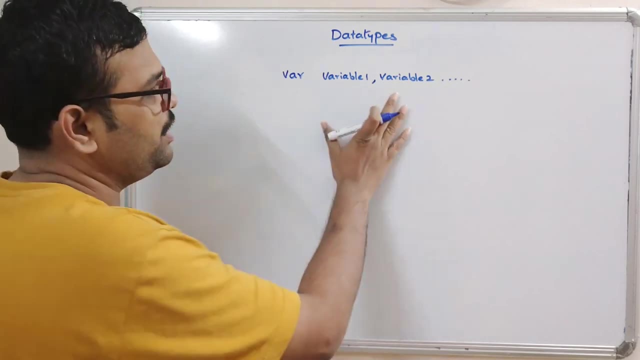 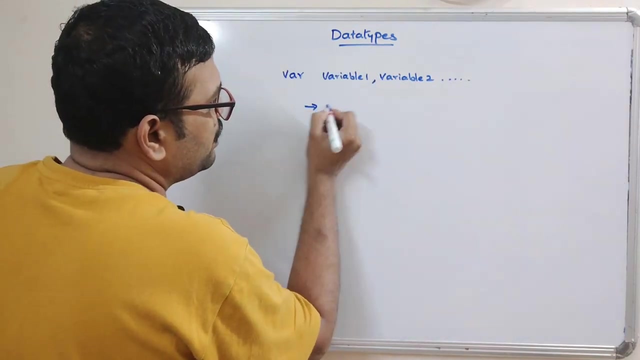 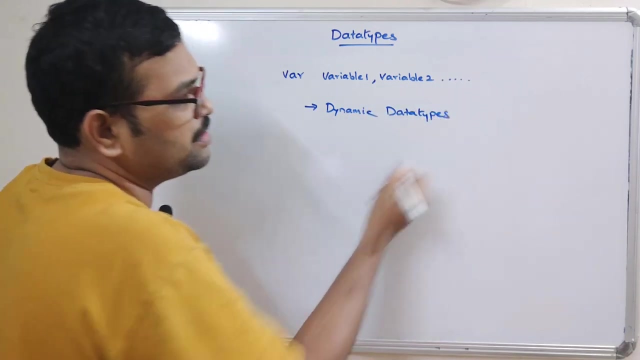 2. Etcetera right. So, irrespective of the data, irrespective of the data, we have to declare the variables using the keyword var And in JavaScript, data types are dynamic data types, dynamic data types. So dynamic data types means based upon the value assigned. 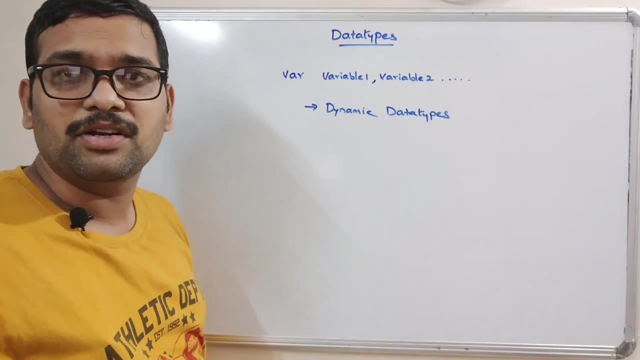 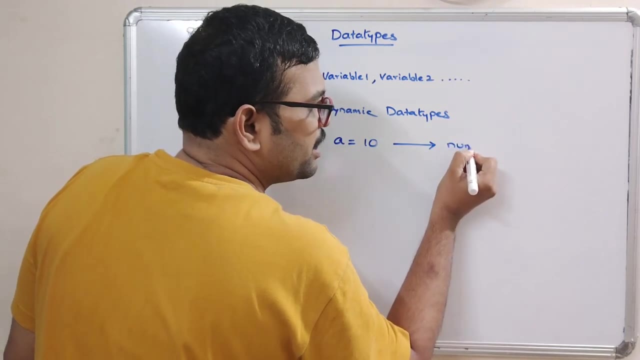 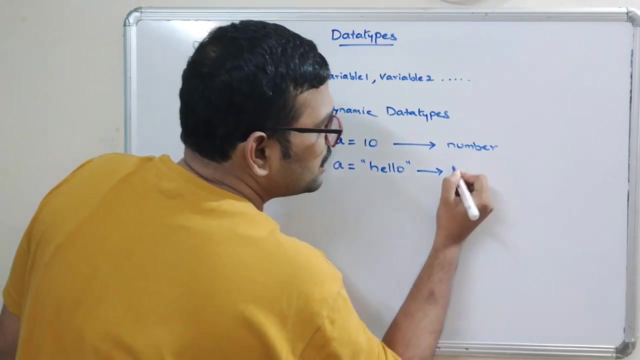 to that particular variable, it will be considered as a particular data type. For example, if a is equal to 10,, this implies it is a number data type. If a is equal to hello, it will be considered as a string data type. So, based upon the value assigned to, 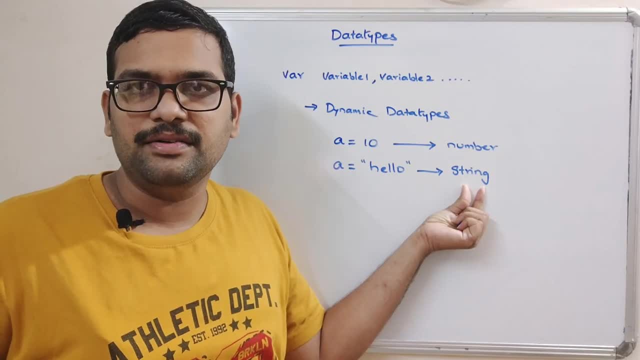 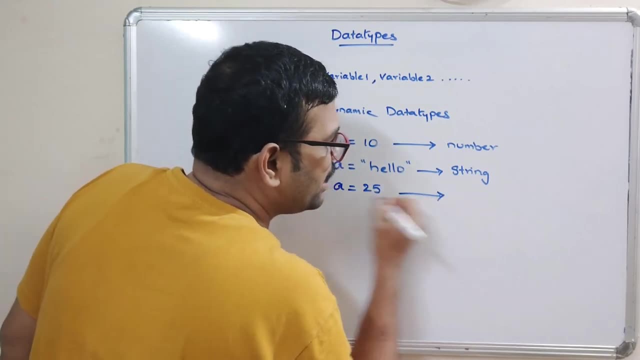 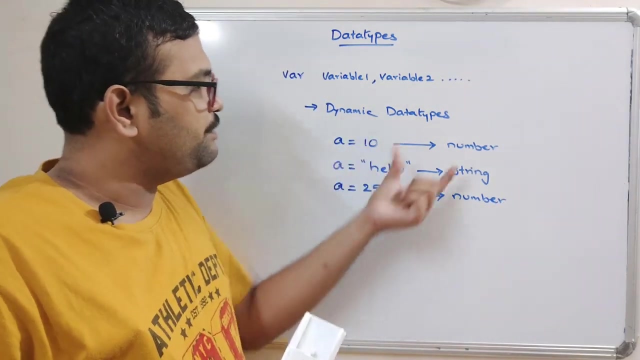 the variable, the data type will be finalized And in an immediate next line, if a is assigned to some 25, again, the data type of a will be changed. So these are the dynamic data types. So we need not declare these variables using the particular data type. So these are the 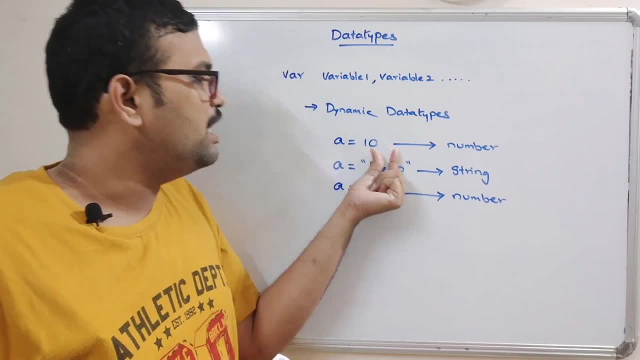 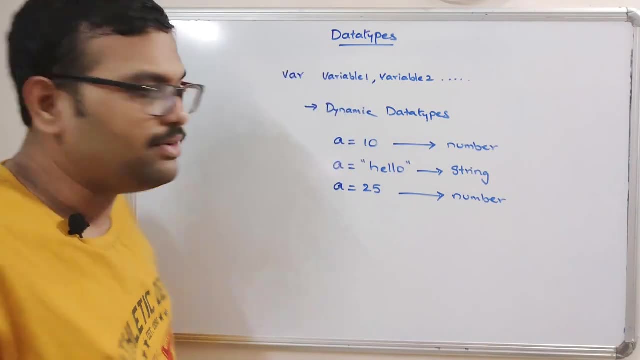 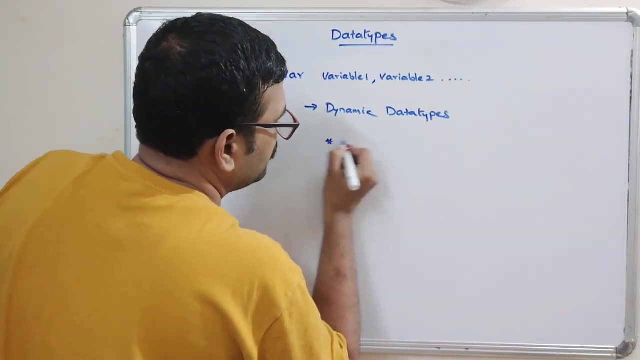 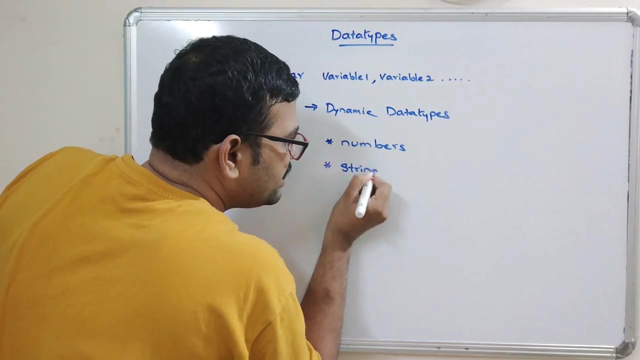 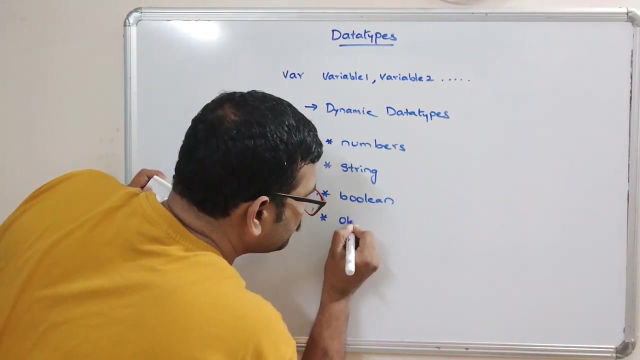 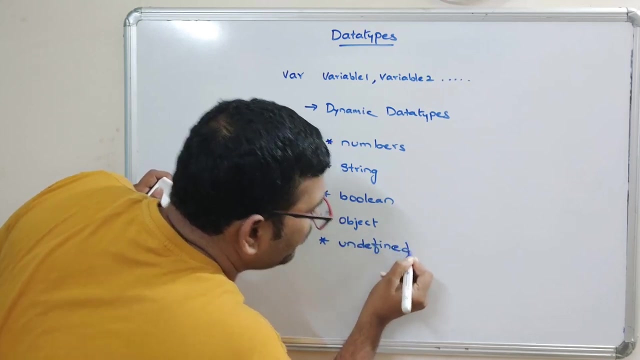 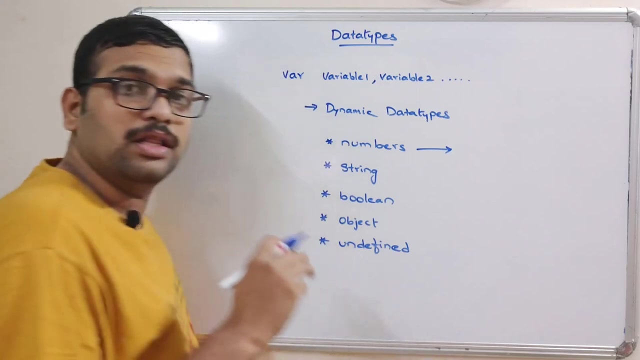 dynamic data types. Dynamic data types mean based upon the value assigned to the variable. the data type of variable will be fixed. And now the data types available in JavaScript are numbers, And I will be string. boolean: object: undefined- undefined. So numbers comes with all the integers and 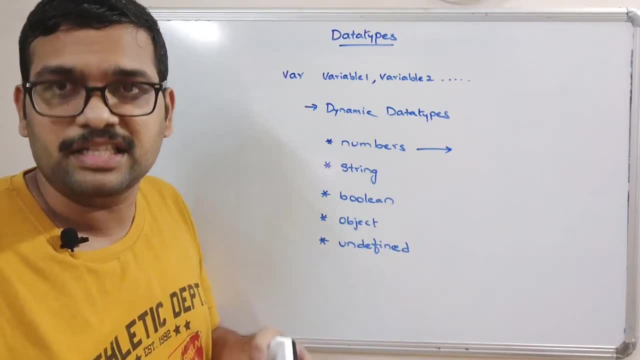 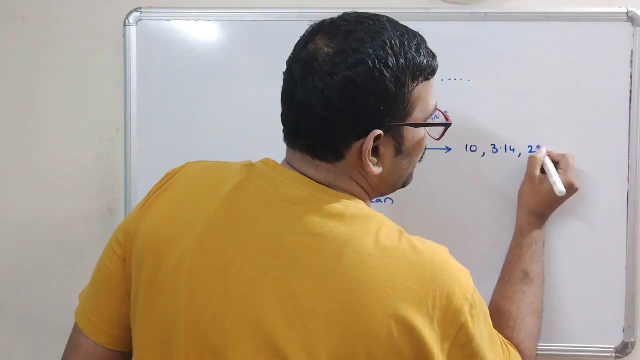 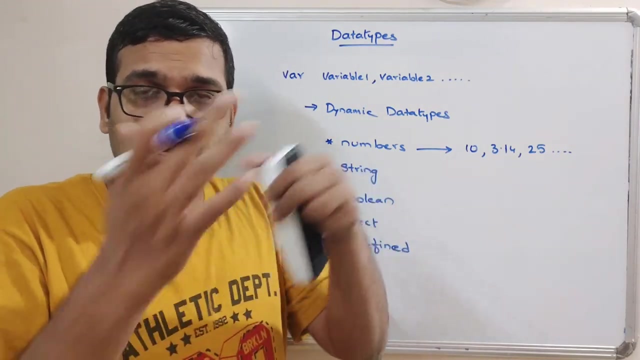 the float values. That means the numbers without decimal points and with decimal points, So for example, 10,, 3.14,, 25, etc. All this comes under the number, So either it can be an integer or the float. So in other programming languages we will differentiate these numbers, these numbers. 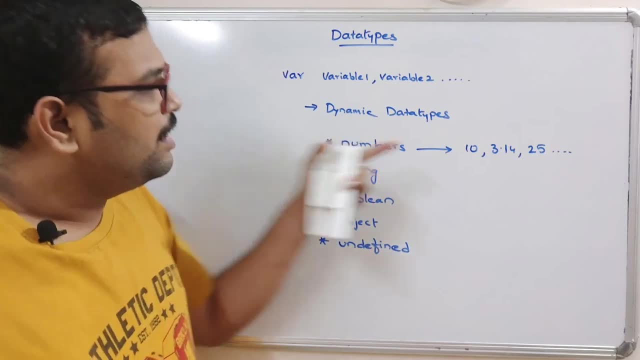 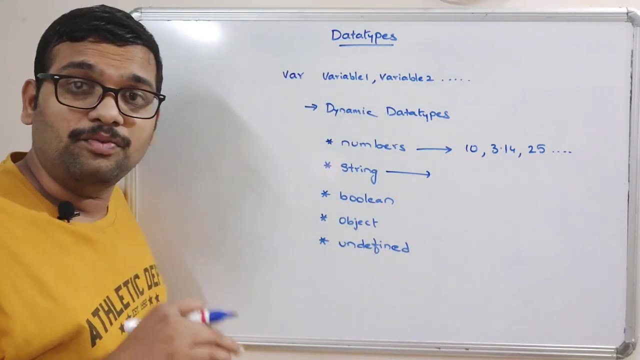 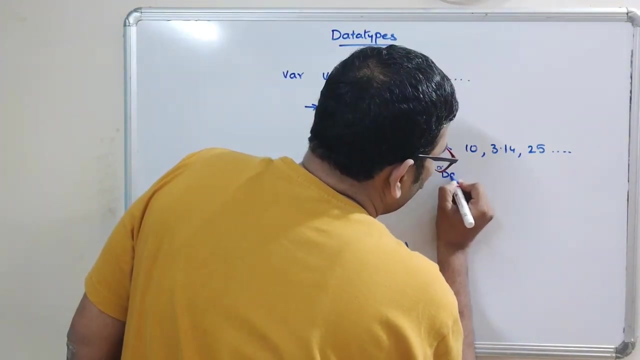 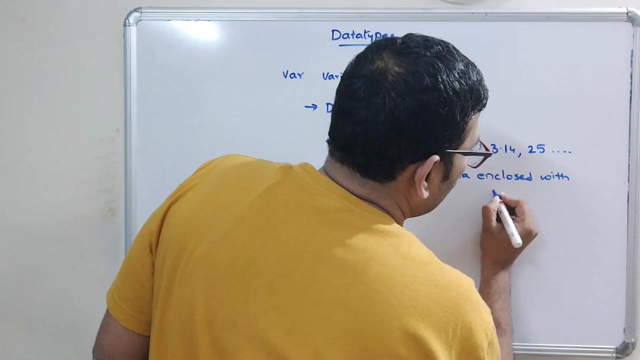 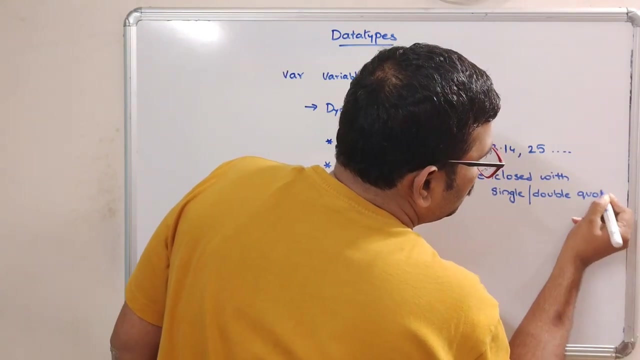 with integers and a float, So, but here everything will be considered as a numbers And coming to the string. So whatever the thing, whatever the thing enclosed in between single quotes and double quotes, So data enclosed with single or double quote, So example. 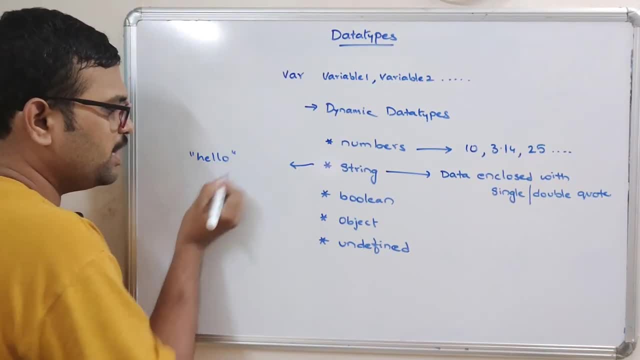 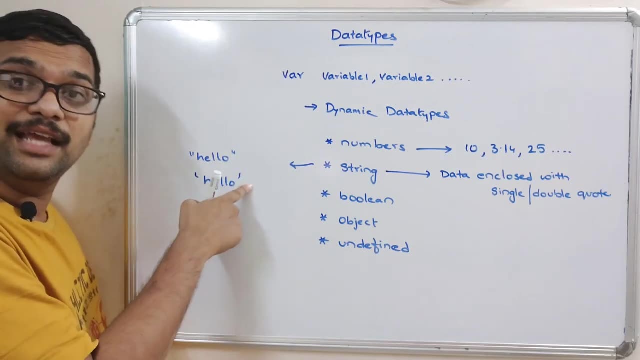 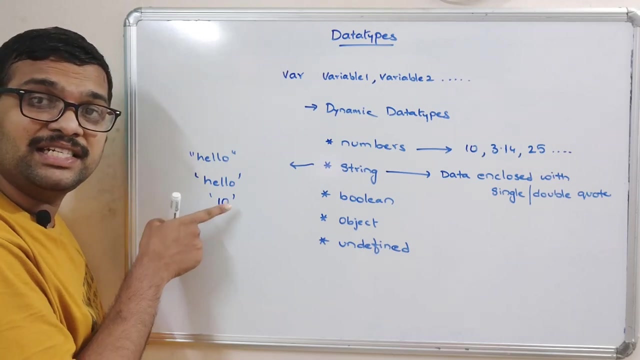 so this is: this is also a string because hello is enclosed in double quotes. This is also a string because hello is enclosed in single quotations. This is also a string. So even though we are giving some 10, but this 10 is enclosed in single quotations, That implies this is also a string. So whatever. 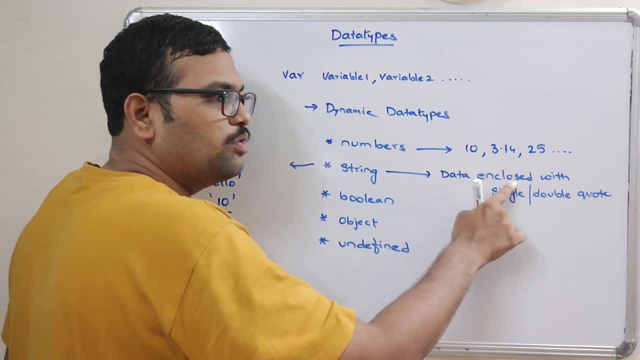 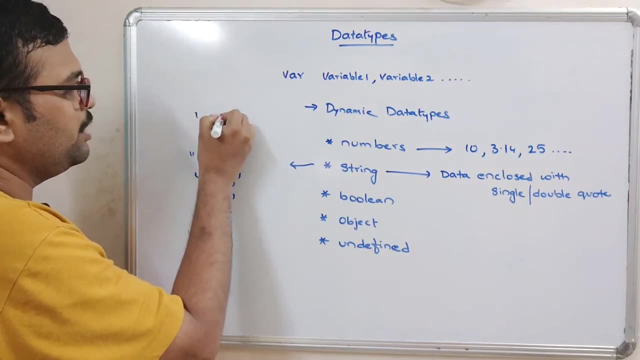 the. so that's why I have written the data which is enclosed with a single or a double quotations. that will be considered as a string. So if you are writing some dollar symbol in between the single quotations or double quotations, that will be also considered. 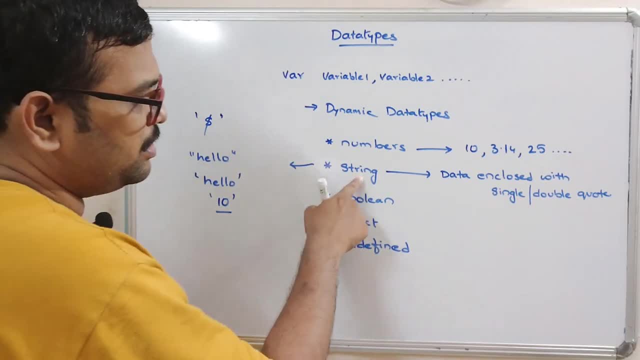 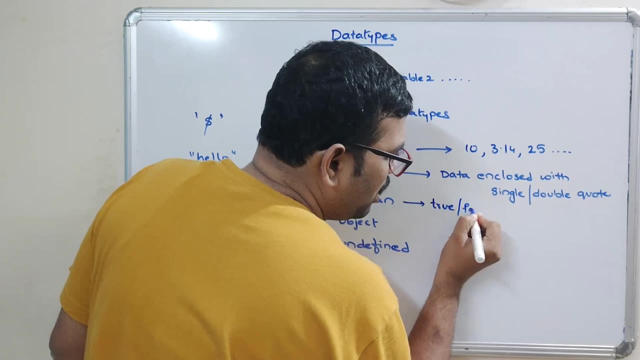 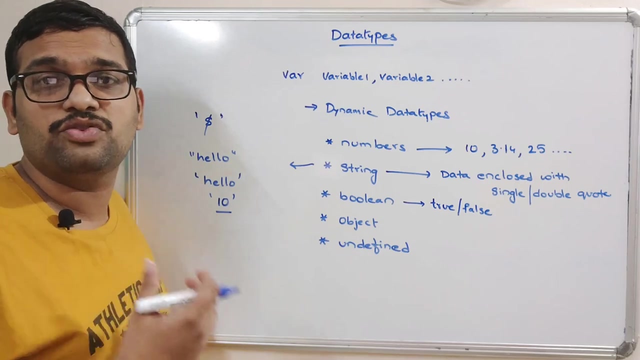 as a string, right. So this is the string data coming to the Boolean. Boolean data type is age through all fields. So whenever we are comparing the conditions, we'll get the result as a boolean result. So Boolean results means either two or all false. So, for example, some age equal to two. 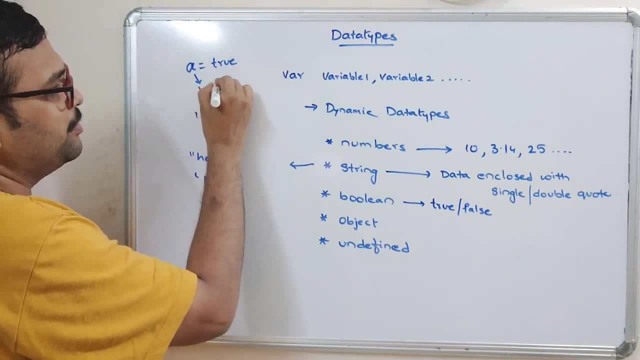 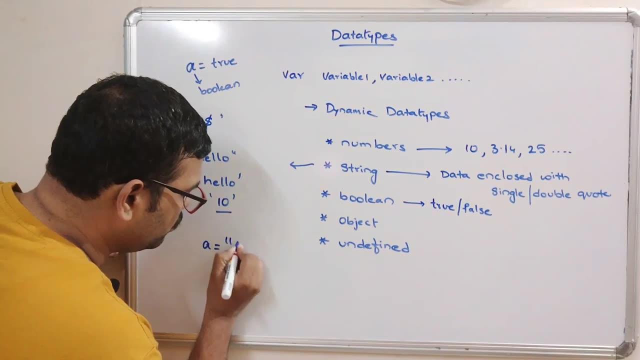 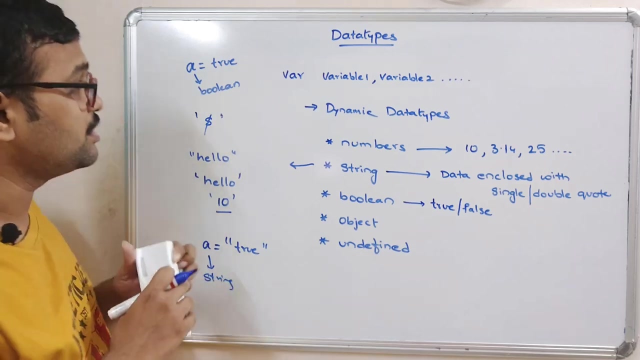 Now the data type of year will be 2.. boolean, now the data type of a will be boolean. if the same thing, written like this, a, is equal to true, in between double codations, the data type of a will be string. that's the difference, right. 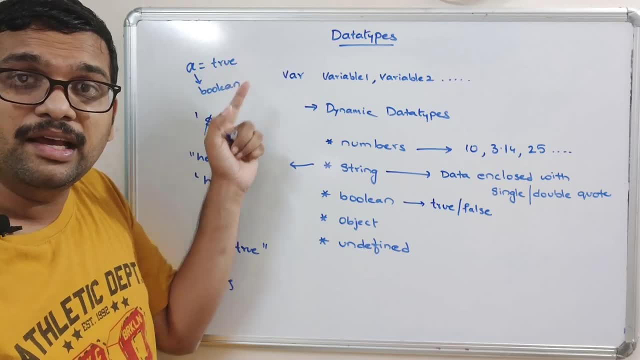 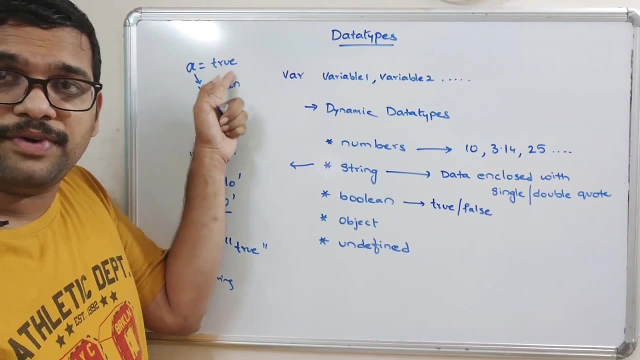 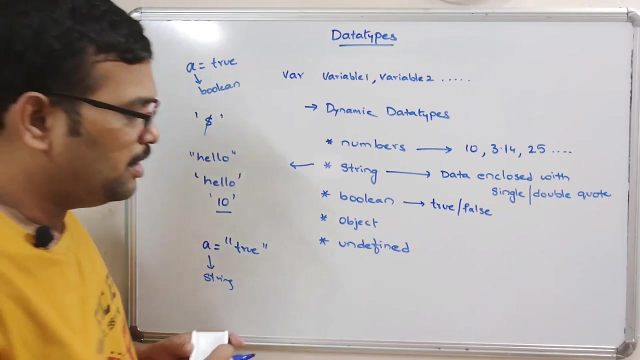 so if a is equal to true, this true should not be enclosed in double codations. that will be considered as a boolean data type or a false or a false. and if the same true or false enclosed in double quotations, then that that data type will be considered as a string data type. and 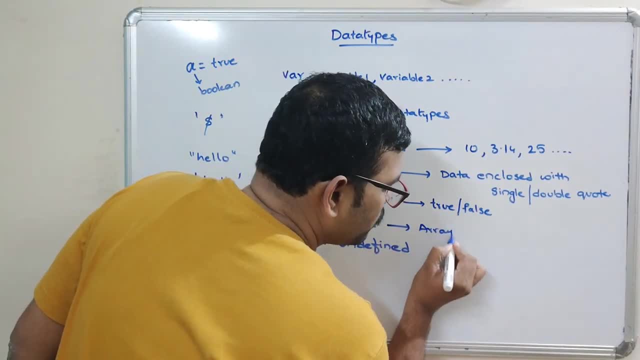 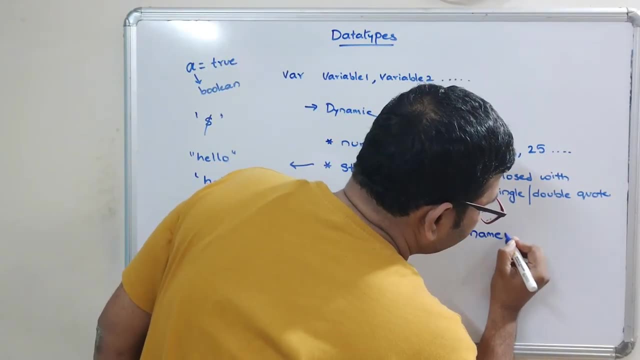 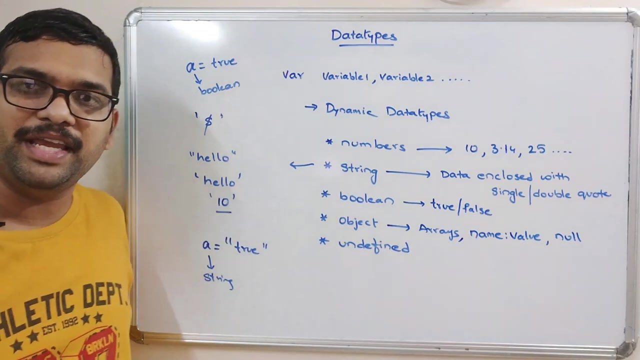 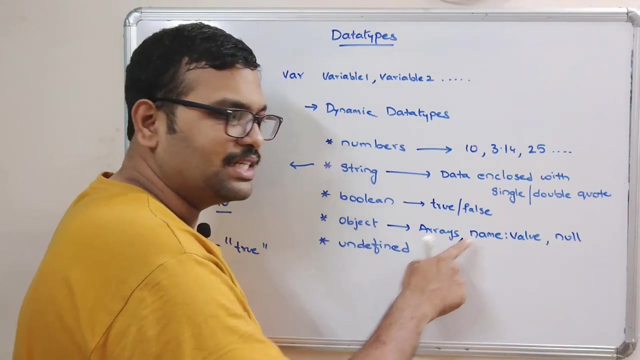 coming to the object, the arrays concept. so the arrays in javascript will be considered as an object, similarly name value pairs, name value pairs. similarly the null statement. the null statement will also be considered as an object. so null statement means if anyone, the object, is initialized to null, that is an empty right, empty- then that null is also an object right. 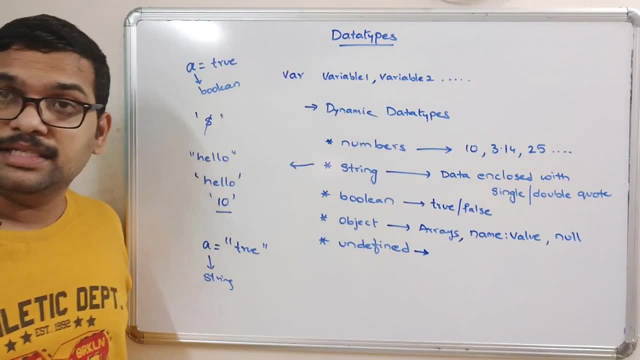 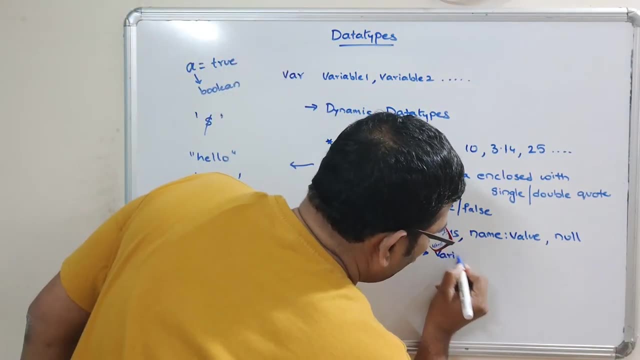 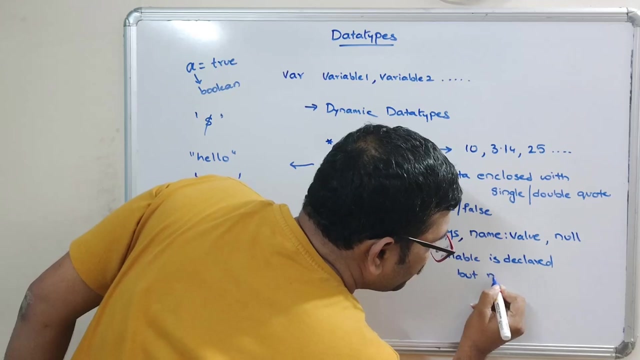 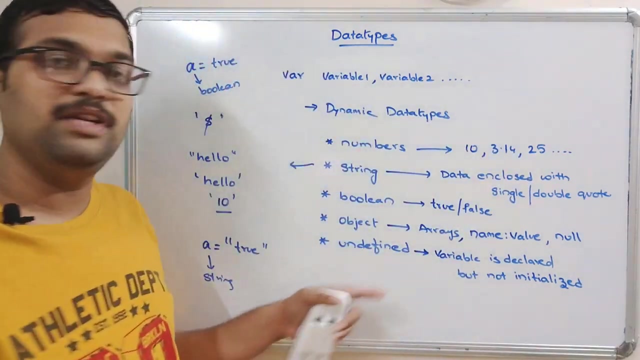 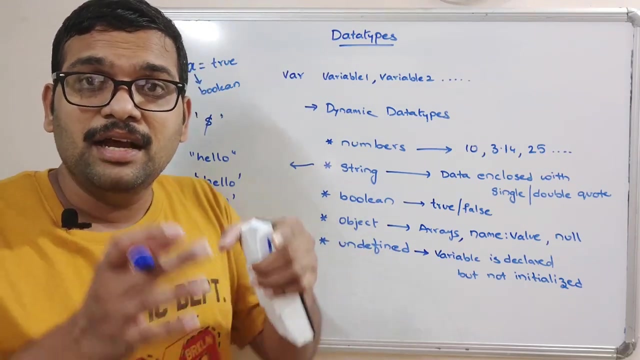 and coming to the undefined, undefined means so the variable is declared but not initialized. okay, variable is declared but not initialized. okay, variable is declared but not initialized, those type of variables will be having the data type called undefined. so unless you assign some value to the variable, that variable 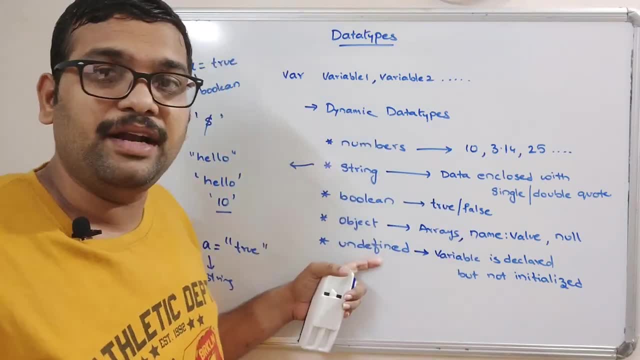 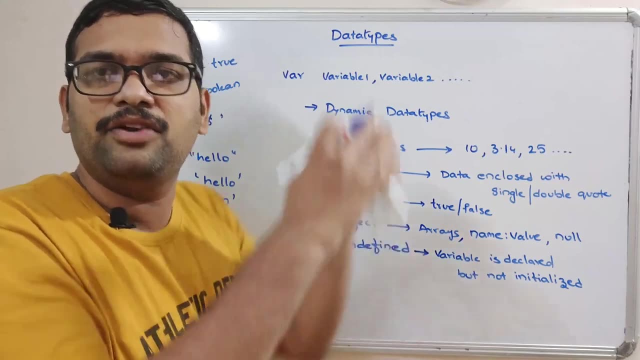 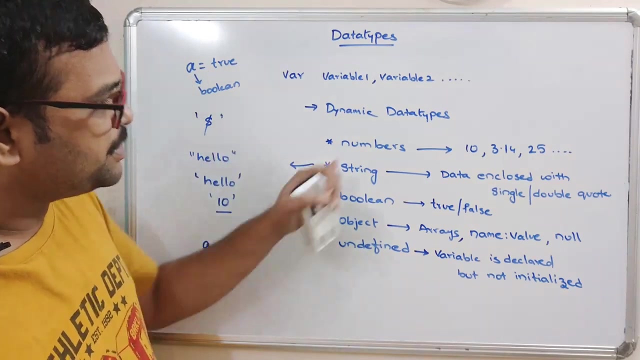 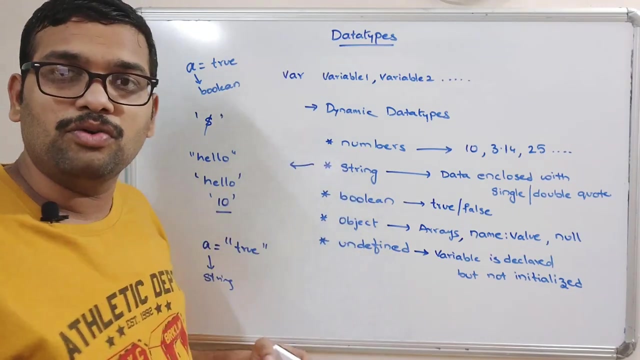 will be of data type: undefined. so whenever you assign some value to that particular variable, that variable will be changing its data type from undefined to the particular value which you have assigned to the variable right now. these are the different data types: never defined numbers, string, boolean, object and undefined. so i will show you on the screen by executing a small 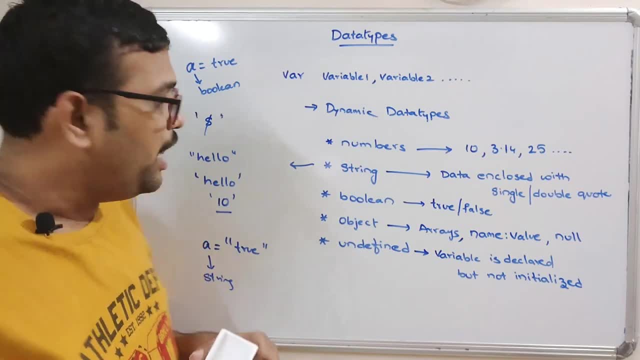 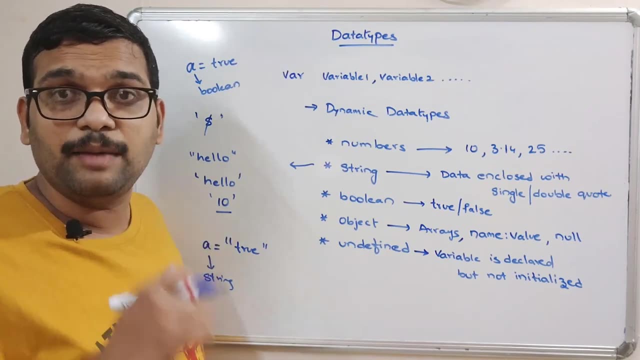 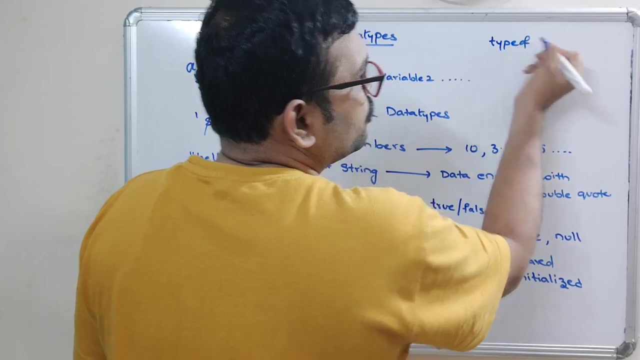 code demonstrating all these type of data types right and how to check whether the particular variable is of particular data type. so finding the data type of a particular variable or a value for that. we are having a keyword called type of. so if you use this keyword- type of- and followed by: 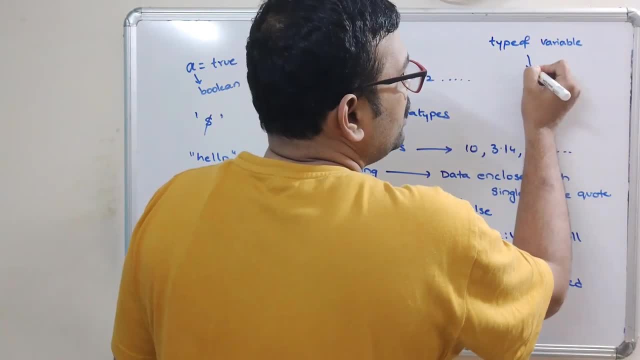 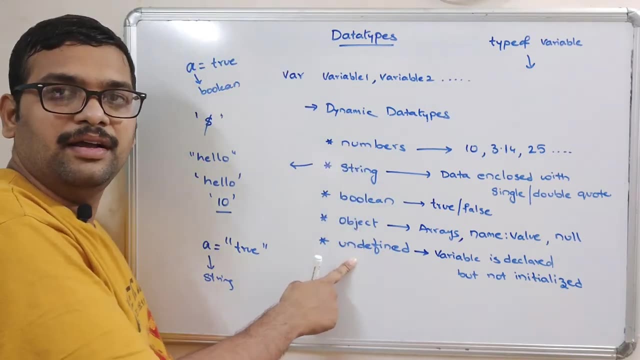 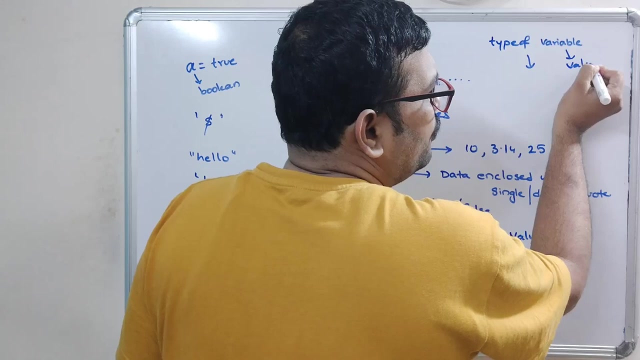 the variable name. this will give the data type one among all these data type- either numbers, a string, boolean object or undefined right. so it will be giving like this. similarly, instead of variables, we can also give directly a value. we can also give directly a value, so you need not go with the variable, you can give. 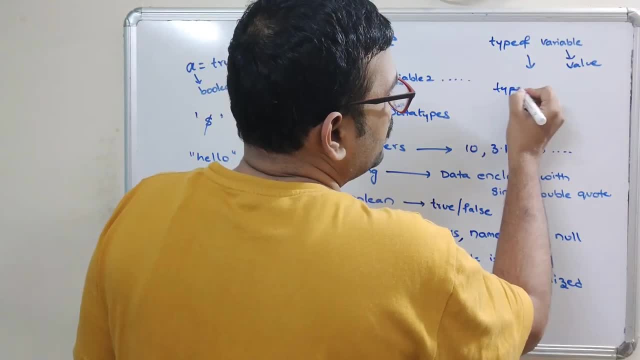 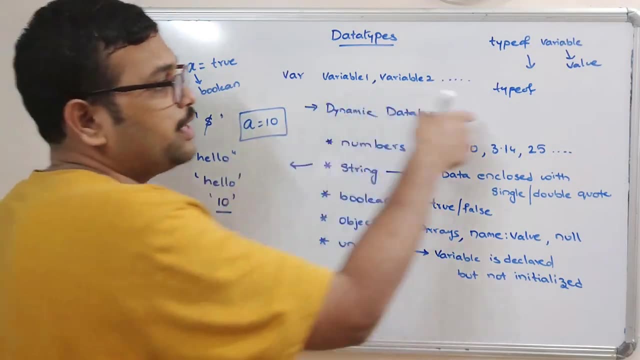 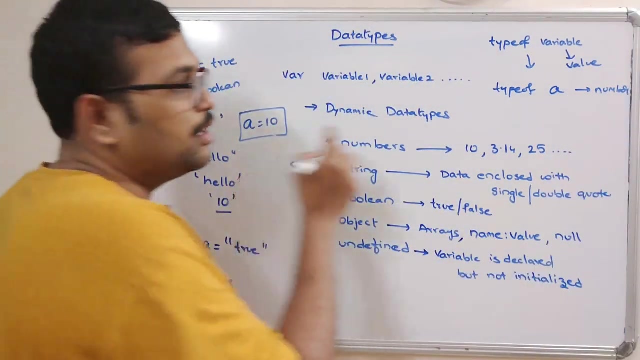 the value. so, for example, type of, for example, a is equal to 10. you consider this example: a is equal to 10. type of a is equal to 10, a. this give a number, the data type as number, because 10 is a number. similarly, you can also: 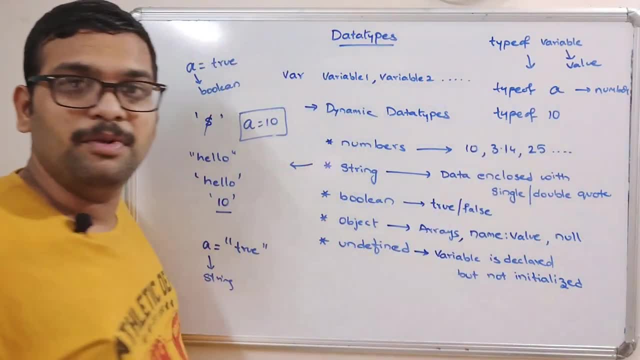 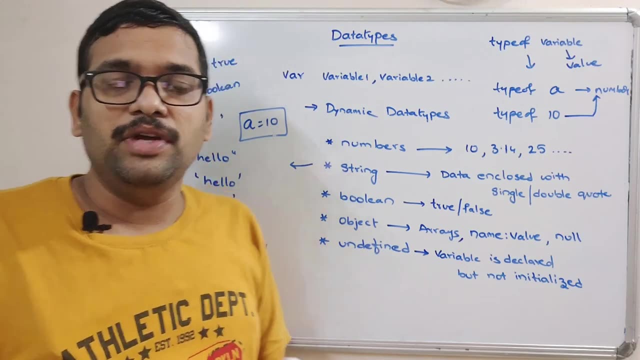 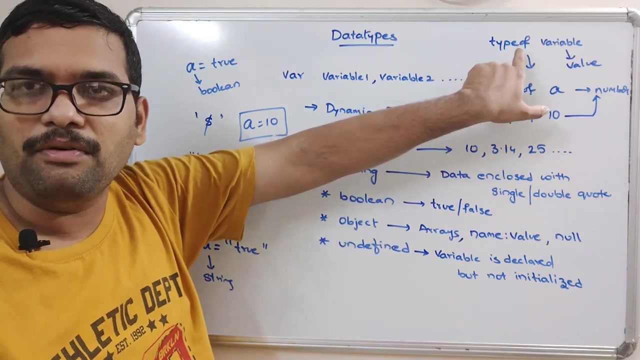 give type of 10, instead of using the variable name, you can also give the value so that it will also give the same result as a number, because 10 is a number, right? so in order to find the data type of a particular variable, we have to use this keyword called type of. you have to use this: 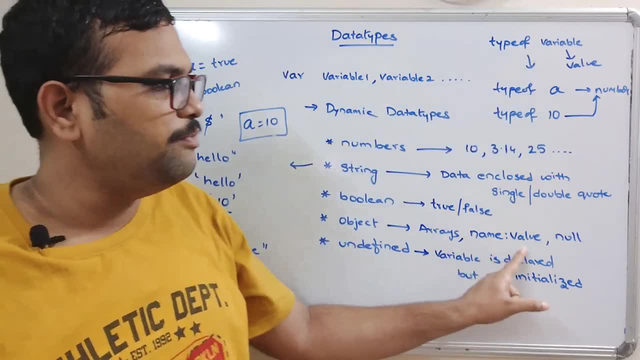 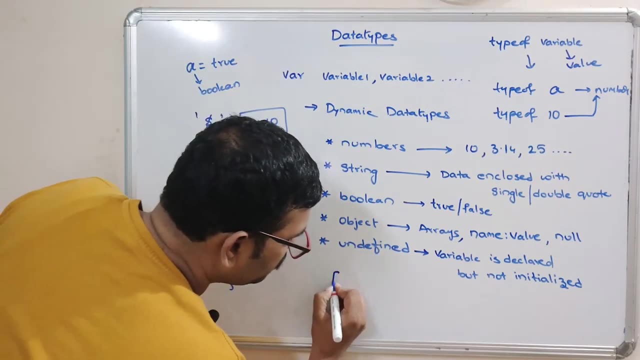 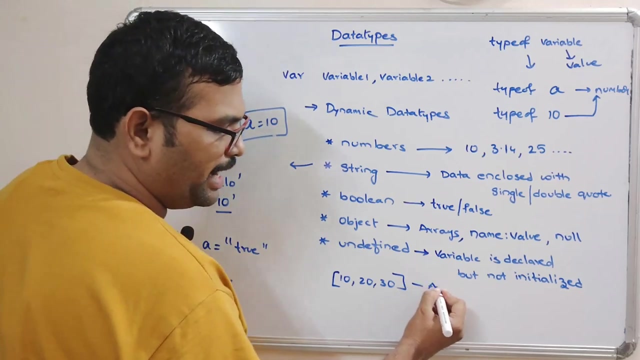 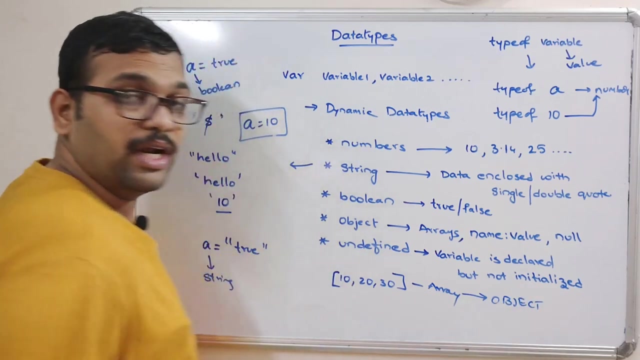 keyword called type of and arrays- name, value, pair and null will be considered as an objects, right? so arrays means we know that. so in the subscript we have to pass the elements 10, 20, 30. this is an array, but here the data type of this arrays is object. this object, right? so i will show. 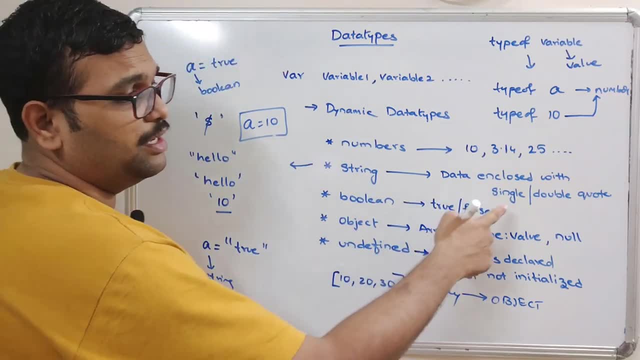 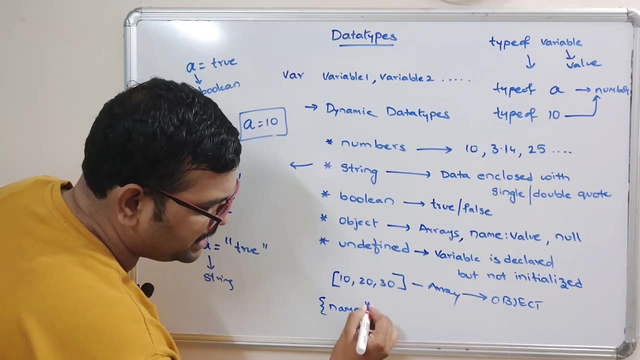 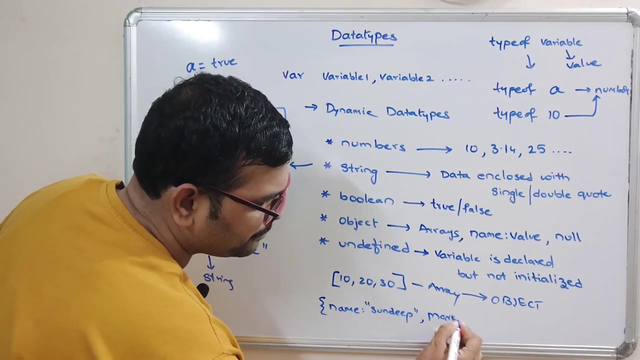 you by executing a small code and coming to the name value pair and null will be considered as an objects, right? so in the subscript we have to pass the name value pair. name value pair so you can give some name, you can assign some name and also assign some marks. so this is called an object. this is called an object, so you can write here. 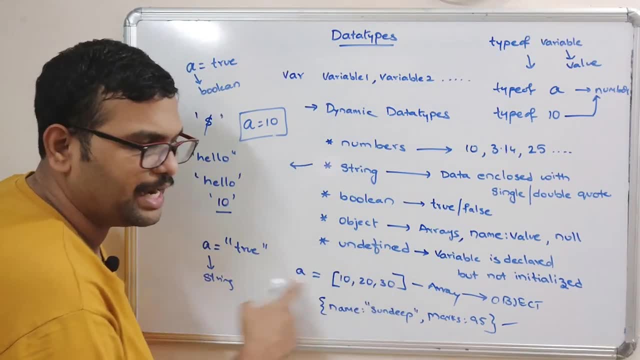 some a is equal to 10, 20, 30. so a is an array which the data type is object, and here the student details or any anything else you can write here. so you can write here: some a is equal to 10, 20, 30. 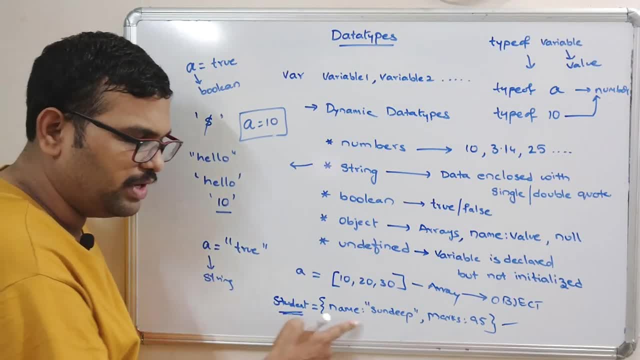 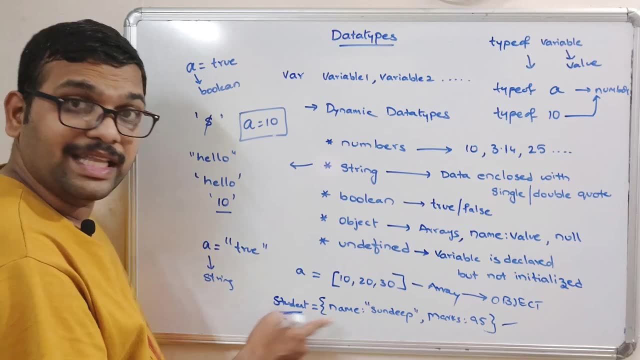 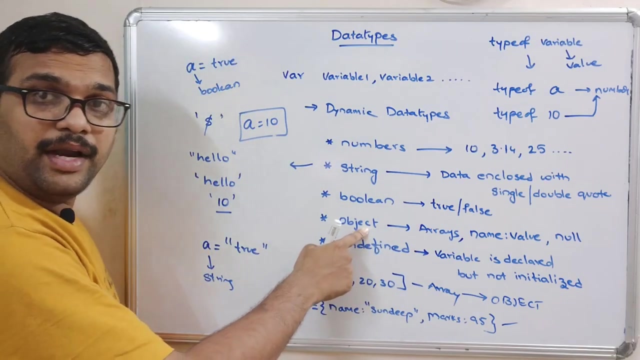 right, so this is a variable. okay, this is a variable. variable is equal to name value pair. so name sandeep marks 95, so student is a object. the data type of this type of name value page will also be considered as an object, right? so hope you understood, all of you, right? so let us move on. 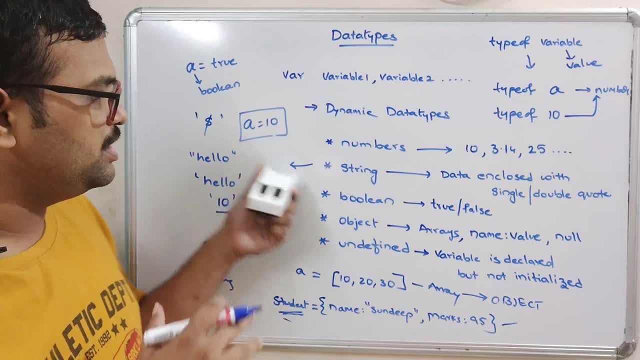 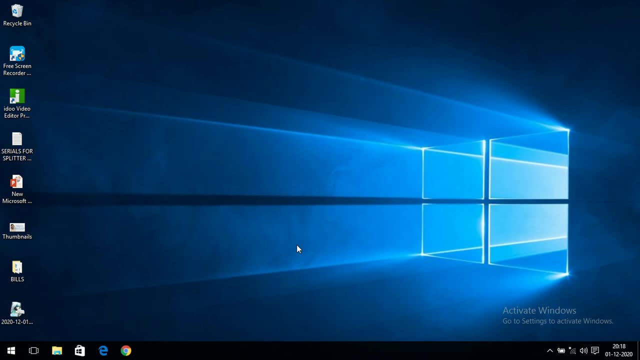 to the system. so i will show, i will demonstrate all these data type by executing a small code. so let's move. hello friends. so just now we have seen various data types available in javascript. now i will show you the demonstration of all those data types by writing some code. so let us open the notepad and 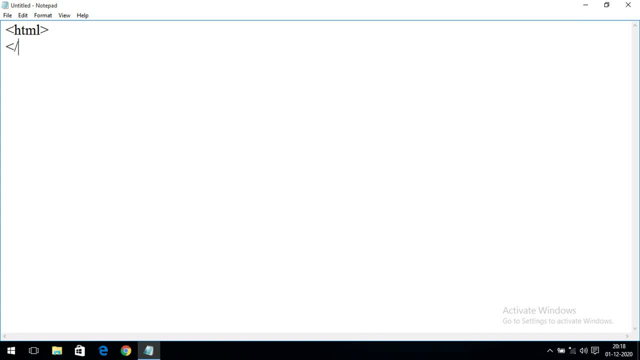 here we will write the script in between the html, in between the html, so as we have, as per our discussions in the previous sessions, so we can write the script in head tag or body tag. so i will write in a body tag, okay, so body and close the body and in between that we will write the script. so in the script again we can. 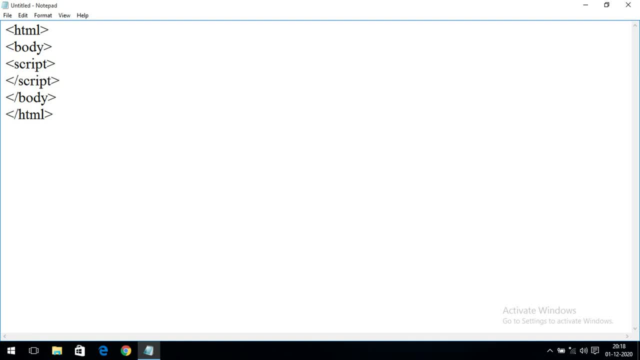 write. we can use a different output options, so which we have seen in the earlier sessions, like we can use inner html or documentwrite, or windowalert, so here we will use the documentwrite to display the output on the screen. and coming to the data types, as we have discussed just now, all 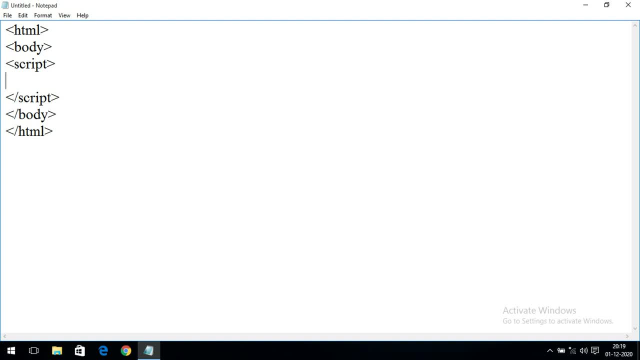 the data types in javascript are dynamic. so we have: all the data types in javascript are dynamic. so dynamic means so, whatever the data we are storing into the variable, those variables should be declared using only one keyword, that is, var, var. okay, so here we have seen the data types like: 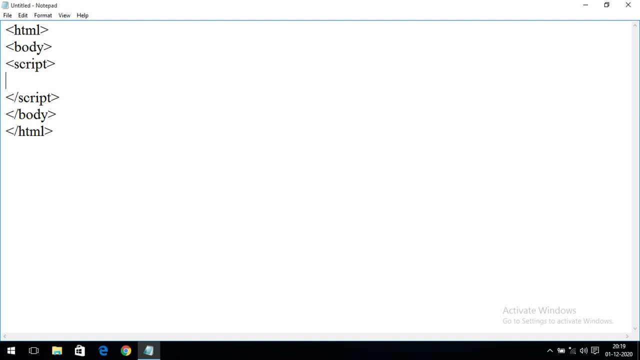 string or numbers or objects or boolean. so whatever the data type, those variables should be declared by using var keyword. so then we can, by assigning a value to that variable, the script will be considered that particular variable as a particular data type, based upon the value which was initialized to that variable. so that's why we call these data types dynamic data types. 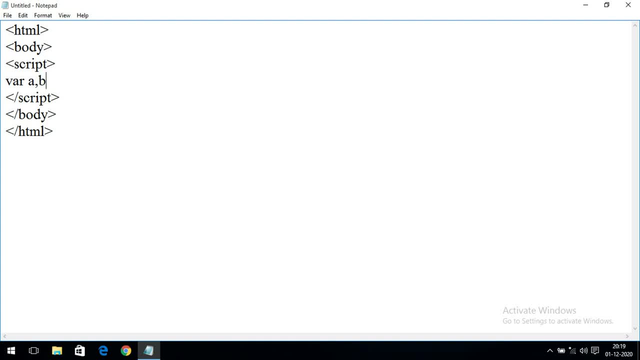 see, for example, i am giving some var a comma b, comma c. that means i have declared three variables. now i am initializing some value. so a is equal to some 10, b is equal to some 3.14 and c is equal to some sunday. so here you can observe. the first a is of integer data type. 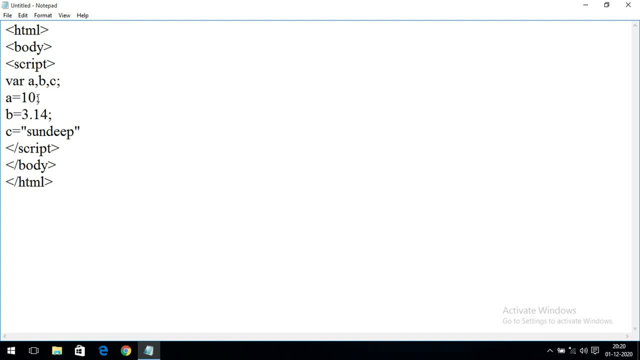 b is also a flow data type, but here we call the integer and float as a common data type called numbers. okay, so here a and b are a number data type. c is an string data type. okay, so in order to check the data type of the particular variable, we have to go with the type of 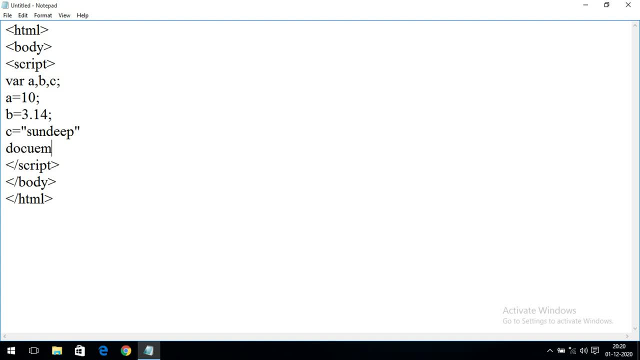 keyword. right, see, we'll see document. document dot write. let us take type of type of a, okay, and we'll go with the talk. sorry, document dot write of type of b. similarly c. okay, now we will check c. so data type of a is just. i am writing here: data type of a is similarly so, just in order to avoid the 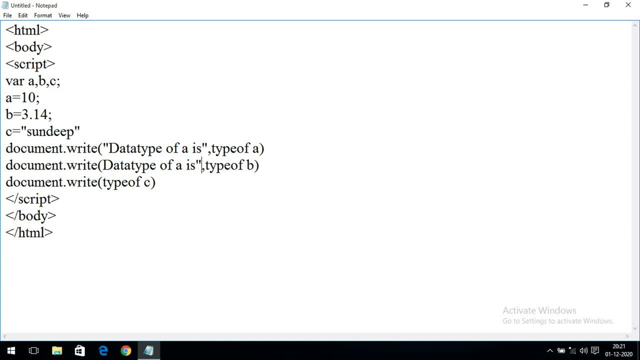 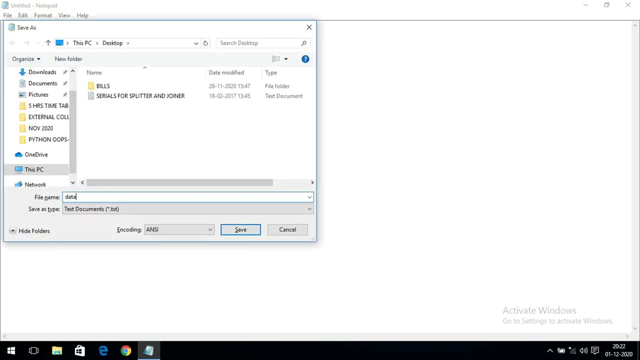 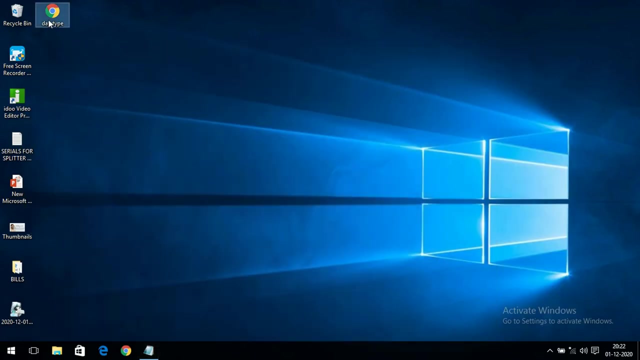 confusions and avoid the confusions, we can write all these things: data type of b, similarly data type of c, so i'll execute this one. i will save this one by using some file name called data type dot. html. so i have saved this one file on the desktop so you can find here. so double clicking on the web browser will get. 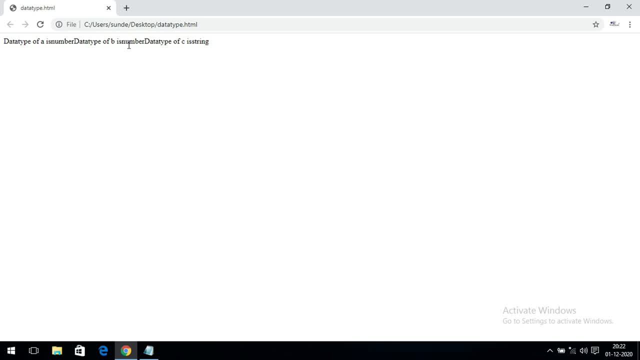 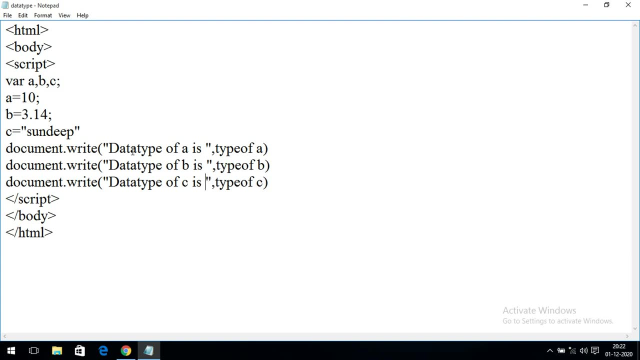 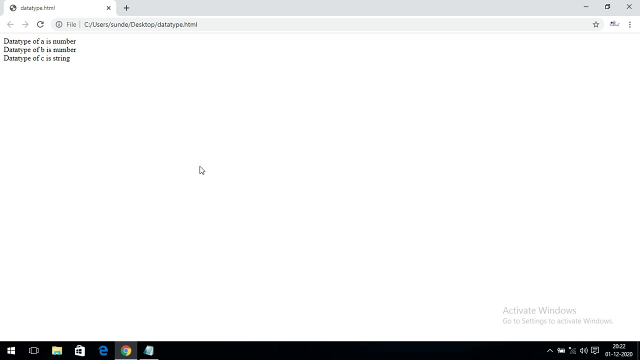 this one. see. so data type of A is number, data type of B is number, data type of C is string. so just give some space here so that it will be displayed here and again. also use the BR tag. so BR means break a row so that everything will be in a different line. okay, everything is. 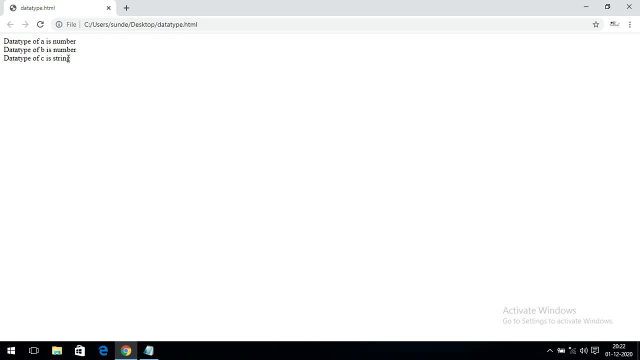 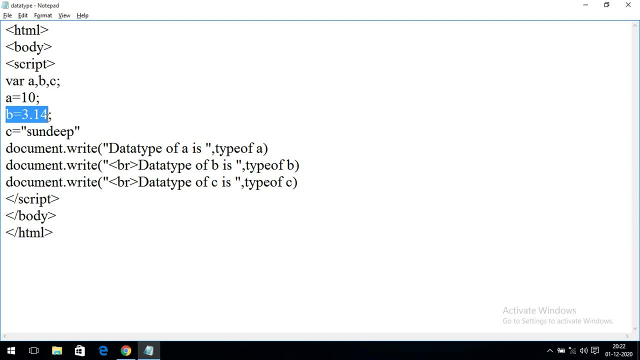 printed in different line. so data type of A is number, B is number and C is a string. you can observe here: A is 10 and B is 3.14. so even though B is having some float data type in javascript, it will be considered as a number. it will be considered as a number and if you write here, see: 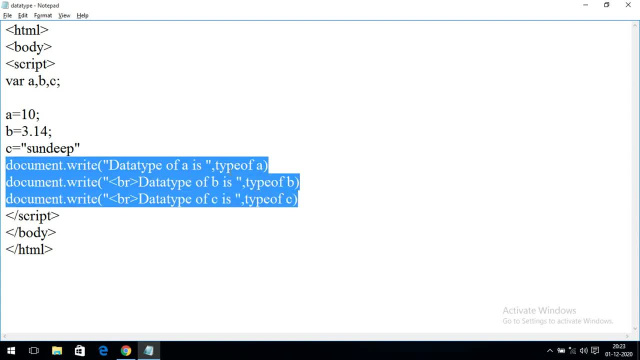 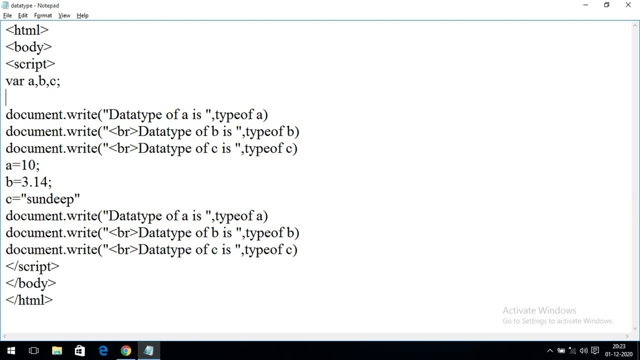 if you write the same thing you here, that means before initialization. okay, before initialization. so I will write here document dot. write: see h1, before initialization, h1, T2 and here after initialization. so we can go with the before initialization and after initialization. see, this is after initialization. now we can observe the difference. so 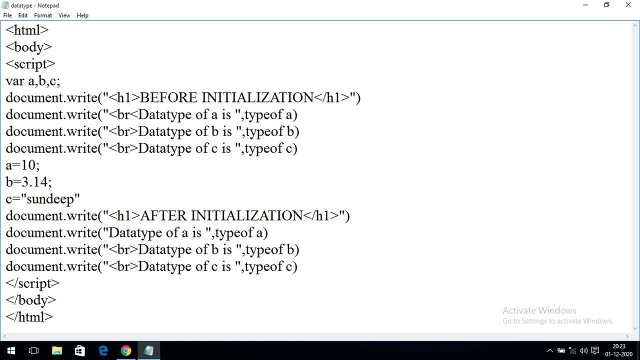 we'll give the break while break row so that everything will be printed in the new line. right will do it here. nowoks, a veer budh, the bi6S opened. so if, alright, all that is just that is good, really. now, here OS is Murphy again huge. he is silent. all right, so now all samples will get. 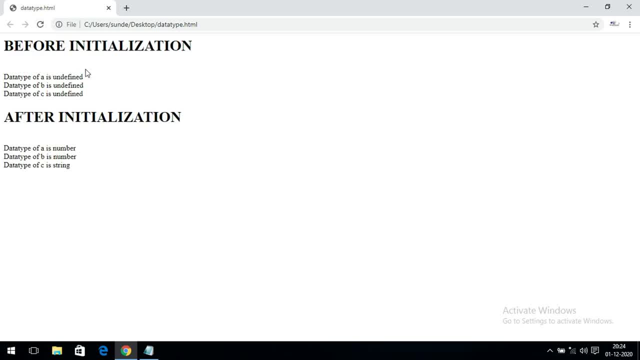 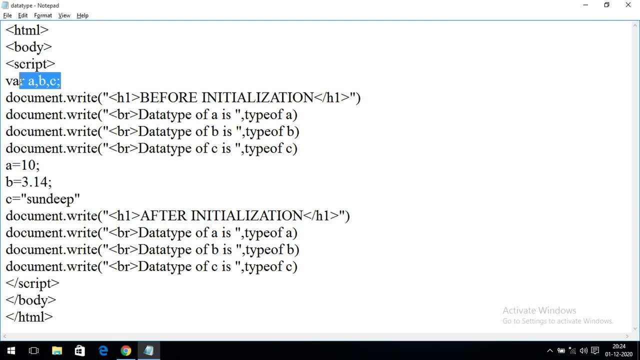 can observe here now- see before initialization: data type of a is undefined, data b is undefined, c is undefined. so if you declare the variables but not initialized the variable, that the data type of these variables will be of undefined because no value was defined to these variables. but whenever we have done the initialization, immediately the variable will be having some 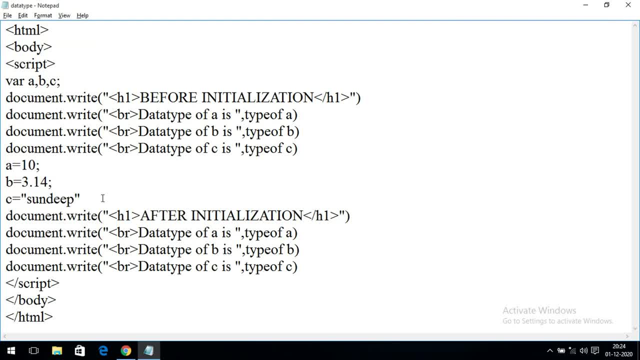 data types right. similarly, let us go with one more thing. where d is equal to true, d is equal to true. now we will check the data type of d. you can observe b is a boolean, so here true is not a string. so if you place the double quotes here, then it will be considered as a string. 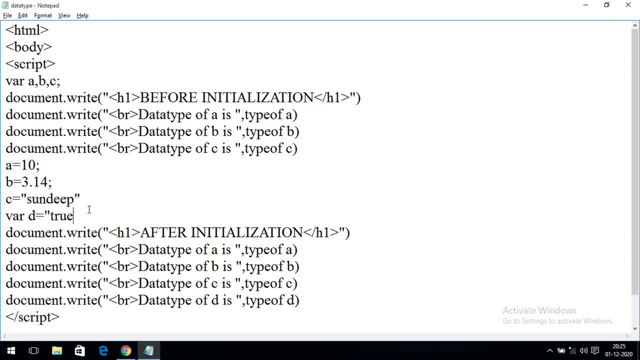 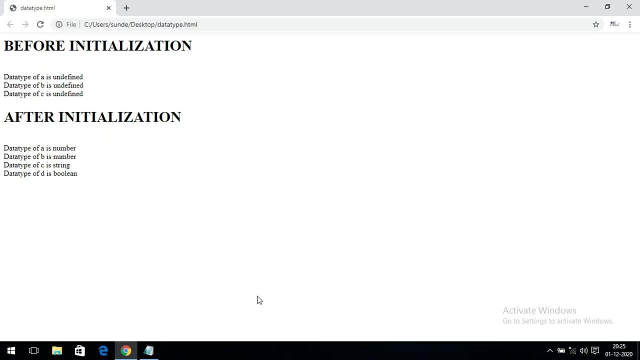 you can observe here now, it will be a string. but if you are not using these double quotations, but you are initializing the value as a true or a false to the variable, to any variable, that variable will be of a data type: boolean. so that's why you can observe here: it's a boolean data type, it's a boolean. 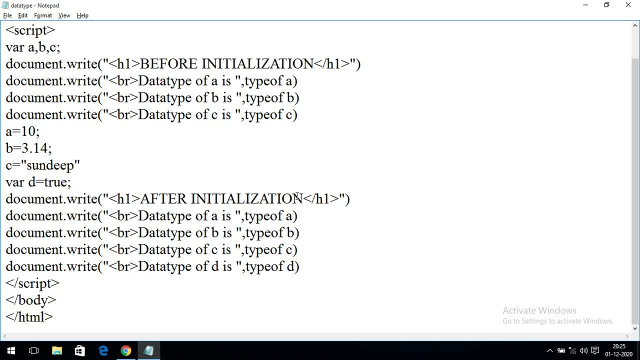 data type. now once again one more thing. so where some marks is equal to right, so some 90, 100, 85, 75, so these are the marks. so here this is called an array. so in javascript this is an array. right, and see where this is. Batman- Nadia Mara. okay, right, here we have some numbers17. 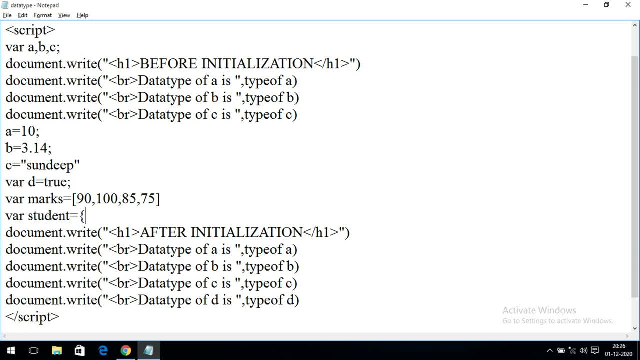 of these, numberhood is also called the parameter name. this is a hunter- the parent number, number, grass method, whatever this can be. we can just take this and we will take method of the method and basically it's just so. that means it's a parameter. so here the function is. 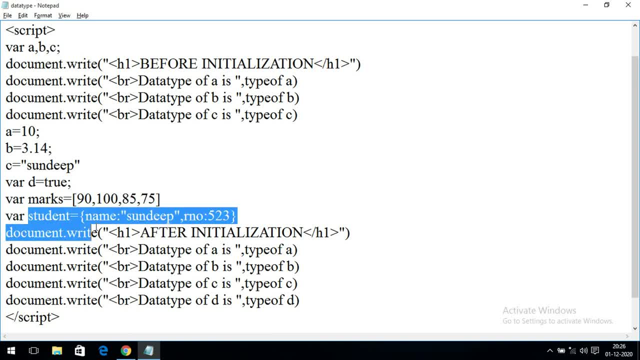 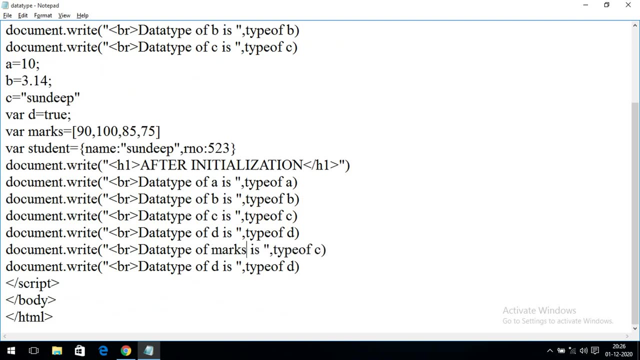 a. you can see that when you start into lesson. I have good object. now we'll see the data type of all these two things. that means marks and the students. see, here we'll see data type of marks and here we'll see data type of student. so here both marks and the student are the variables, right? so 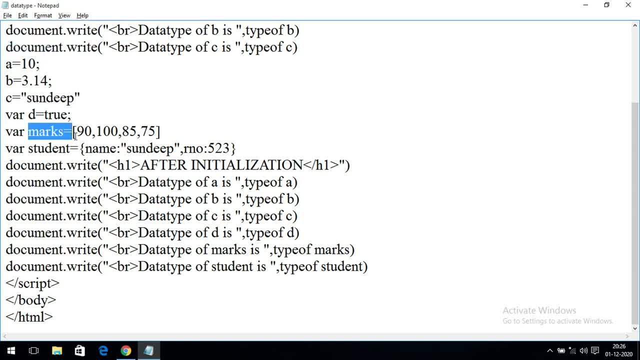 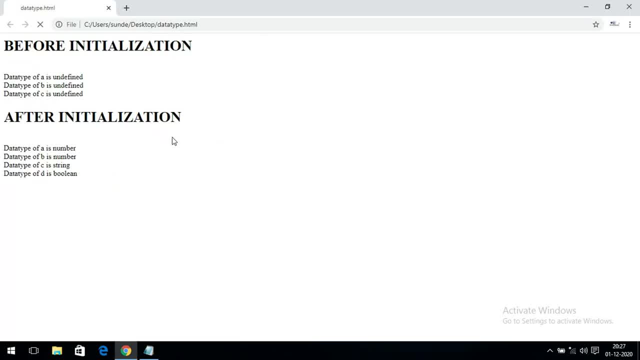 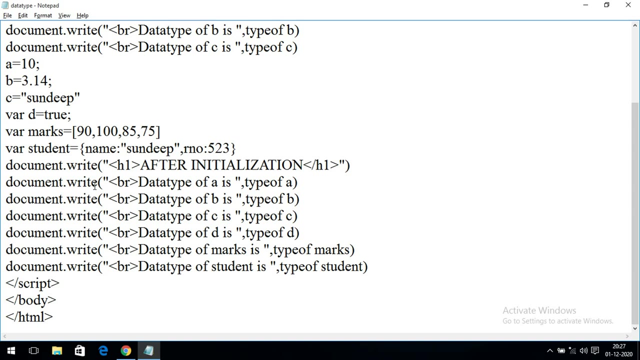 here. we can get here in JavaScript, even though it is an array, the data type of this particular array will be of object. see, you can observe here: see: the rate of marks is object. data type of student is object. right, so this is the one more data type in JavaScript that is an object, so we can declare any variable as. 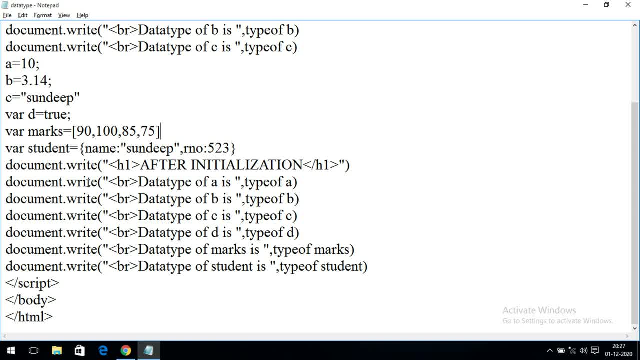 an object. object means multiple elements. okay, so we can use a name- i mean the key value pair, the name and value pair, as well- as we can also assign the arrays concept. so if you are using some arrays concept, also the data type of this array will be. 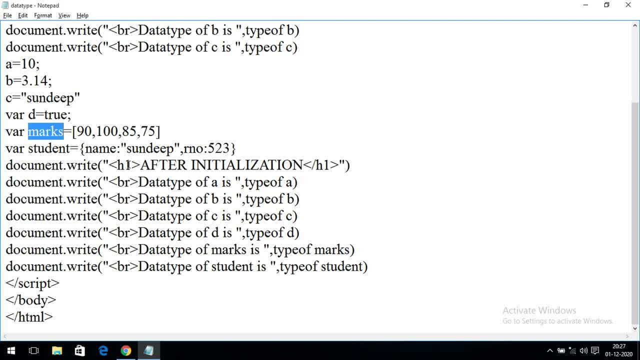 an object. right, so you can initialize or you can uh, reinitialize this object to a null. null is nothing. okay, null means nothing. so if you go, the student is equal to null, null, so immediately we get it as a null. okay, here null is also an object. null is also an object. that means it will empty. 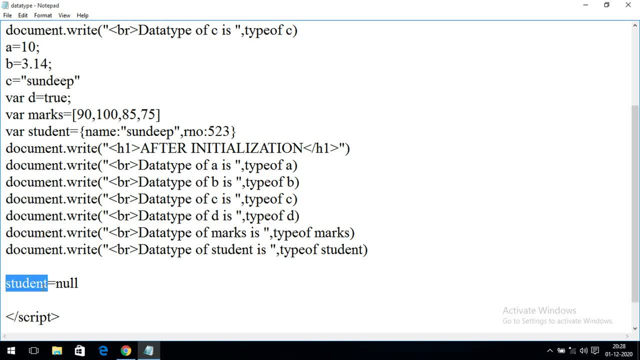 the values of particular variable, it will empty the value of that particular variable. so you can, you can observe here: so the null is nothing. so if you go, the student is equal to null. null is also an object. so if you go, even though it is a null, it is also an object. so data type of null. so here we can directly. 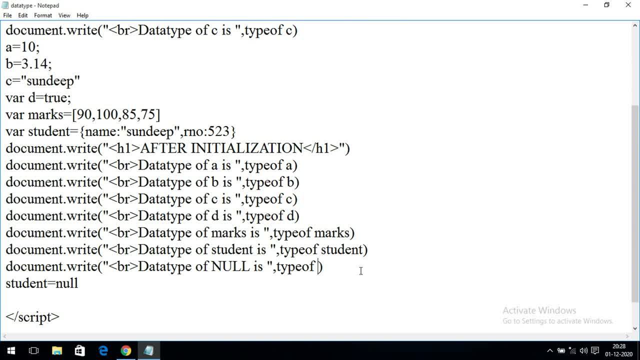 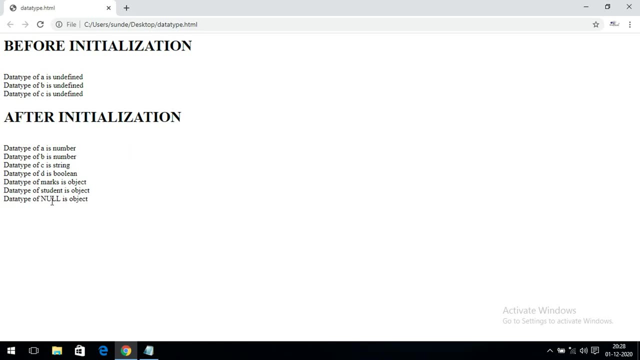 give the value. so two things can be done. so if you use the type of, so you can give either a variable or the value. here i will give the value as null, small letters, null. so let us check. you can observe the data type of null is also an object. data type of null is also an object. 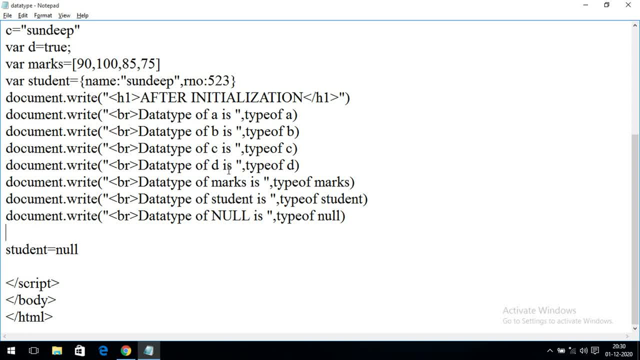 all right. so if it is an, these are all the data types- different data types- and if you want to access the array elements, similar to our other programming languages, we can access the elements of an array by using the index values. here also, the index will be starting from zero, right? so if 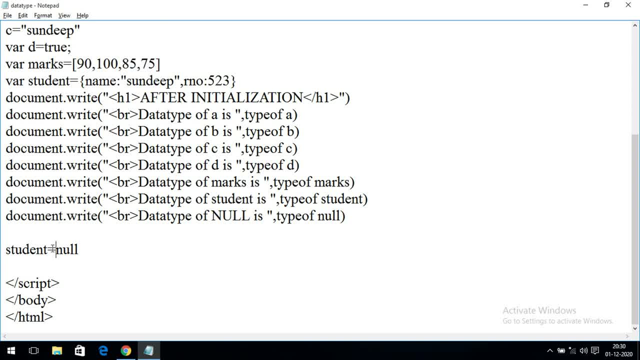 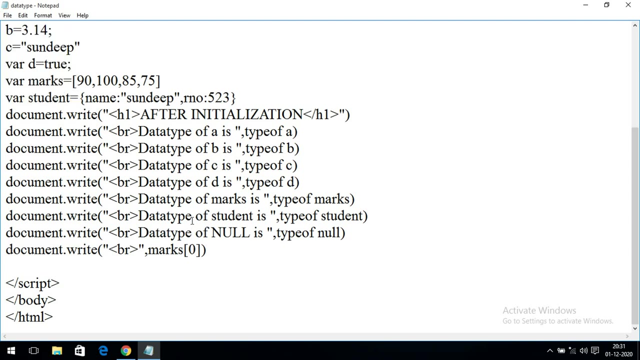 you want to access these array elements, so directly go with this one. so document dot write dr, dr, dr, dr. so marks of zero. see, you can observe here the marks of zero is 90 right. similarly so marks of three. so that means the zeroth index, first index. 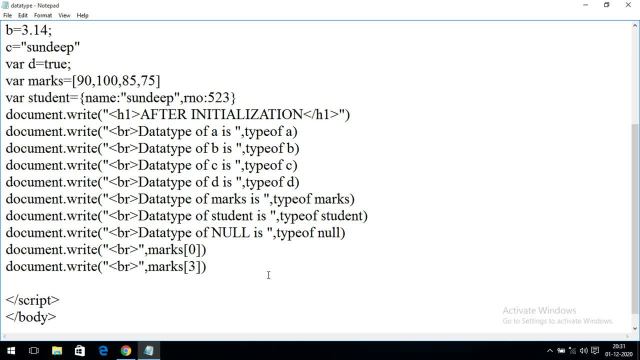 second index and the third index, so marks of three. it should be up in 75, so 75 will be there right? so this is. this is the way we can access the elements of an array, if it is an object. see if you, if it is an object here, and how to access these elements so similar to our structures. 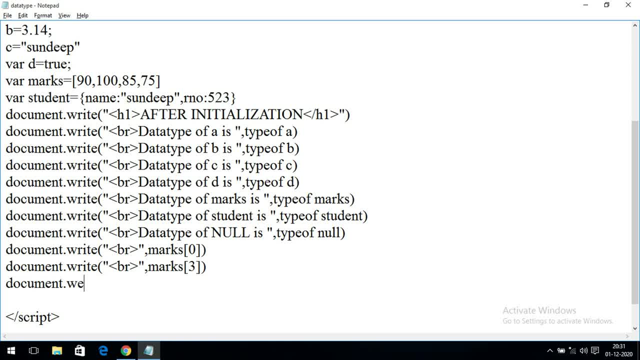 concept in c language. so document dot write, and if you want to access the elements of an object, so simply use the variable name. so here we can say that the elements of an object are here, so we can. variable name: is a student dot the name. right, student dot name. You can observe here it will. 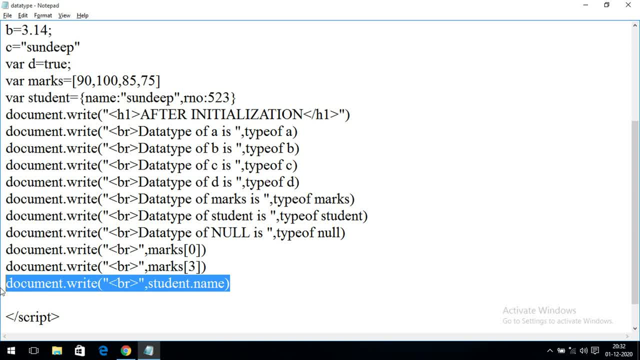 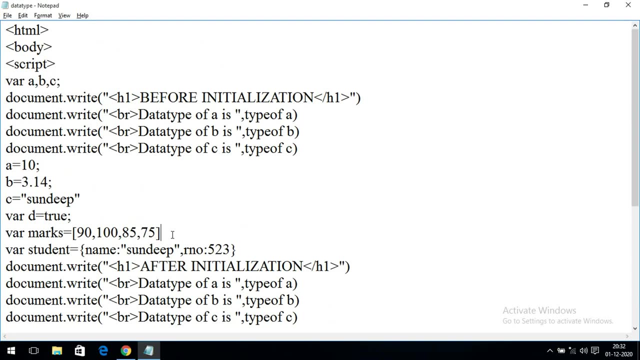 be displaying the name of the object. Similarly, if you want to get the roll number, simply go with the r number, So directly we will get the result as r number. ok, So here this is an array, but the data type of this array is an object and this is an object. and this is a boolean and this one is a. 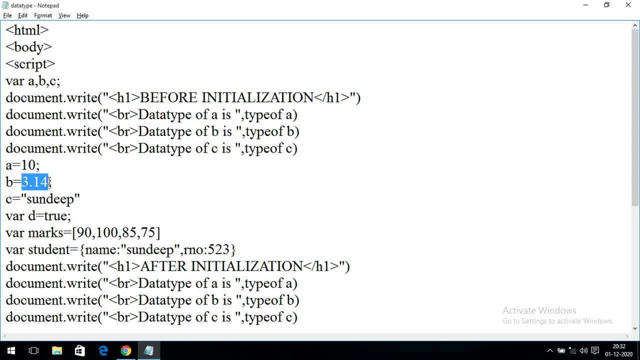 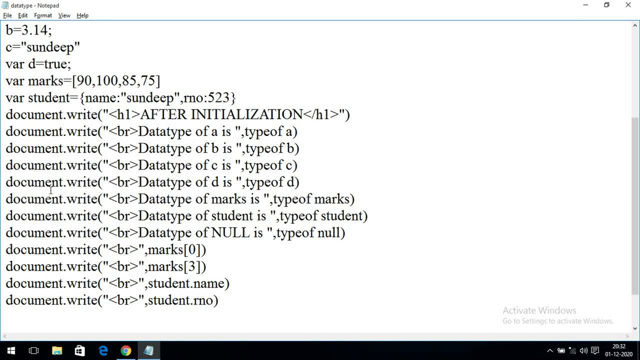 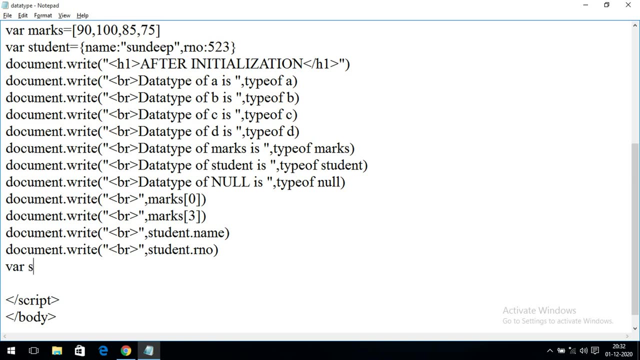 string and this one is the float, but the data type of b is a number. here this is also a number, and also we can represent the string in either single quotations or double quotations, So both we can use. So I will show you So where s1 comma, s2, two variables, I have given two variables, So we can. 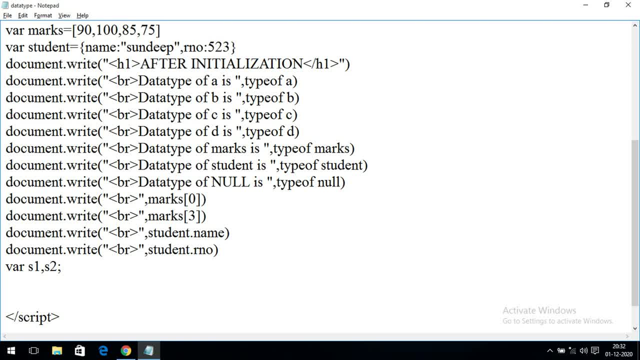 assign any value. any data type of value can be assigned to these two variables. So now I will go with. the s1 is equal to. in the double quotations I will write: yours. So I have given apostrophe s right, yours apostrophe s. So that means I am using some single quotation here. 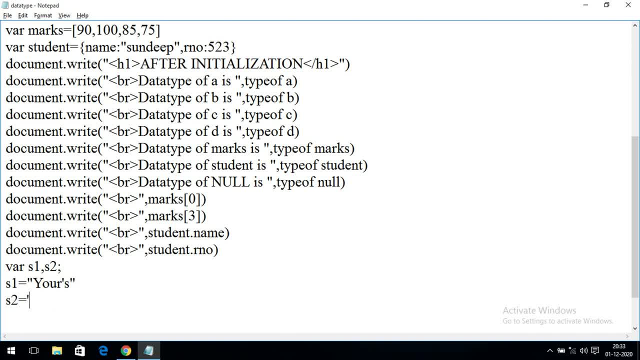 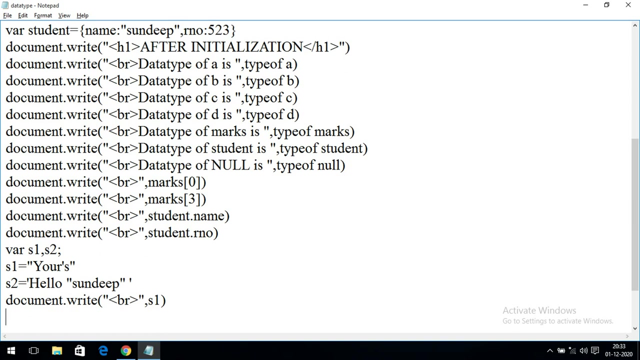 and similarly, s2 is equal to single quotations. hello right. So inside the double cotations I have given some single quotations. right Now I will print documentwriteS1. similarly, document filming- right with us. best loan to me: document dot. right, we are s2.. So inside the double quotations I have given some single quotations. right Now I will print: document Write- v s1.. Similarly, document write: WE are S2. 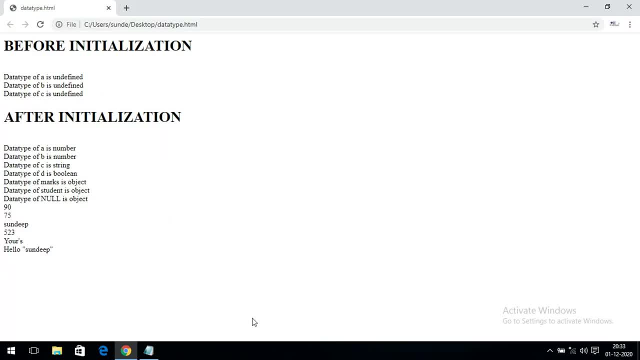 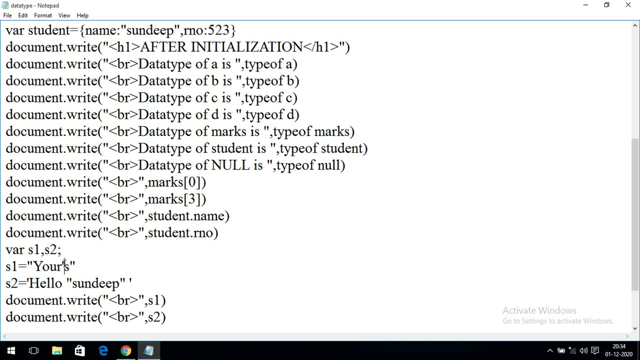 you can observe here- see inside the double quotations, we can use the single quotation. inside the single quotation, we can use the double quotation. right? so here you can observe, we have given the complete content in double quotations. inside the double quotations we have given one single quotation. but that has been displayed on the output stream. and coming to the second example,